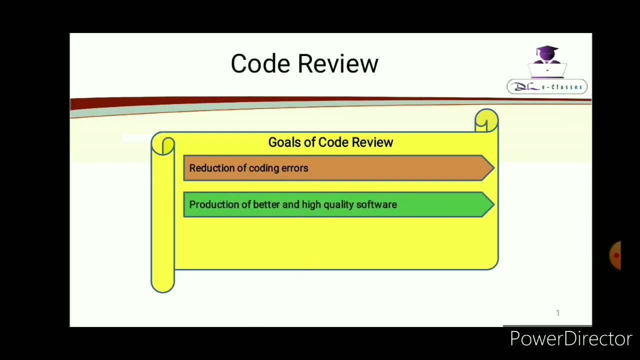 to reduce the coding errors. production of better and higher quality software. finding better solutions for a software product, development strategies. Now, this means, when you do coding software development strategies, you are not just doing the code review, you are also doing the code review properly. Then, if a particular solution for a particular software product 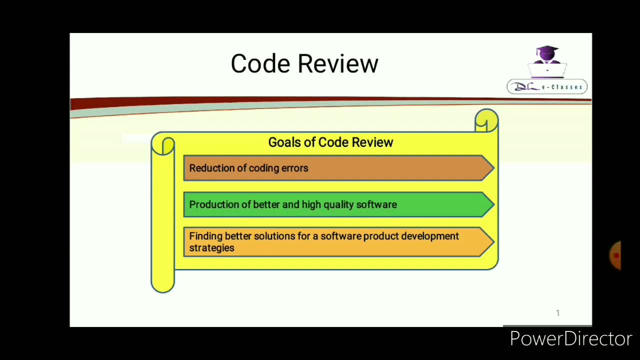 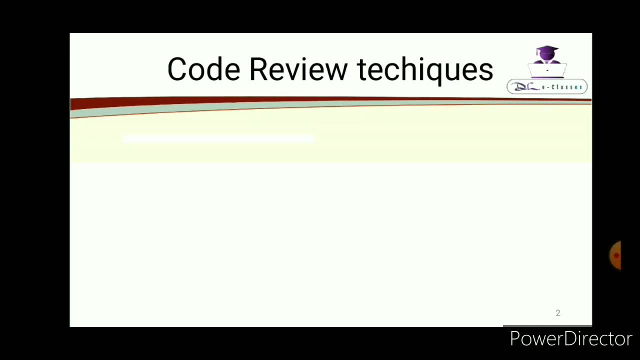 development strategy fails, then you cannot choose or find out alternative solutions for the particular development process. Now, when you are talking about a code review, there are different types or different classes of different scope of code review techniques, But overall, the code review techniques can be classified into two types. The first one is known as the 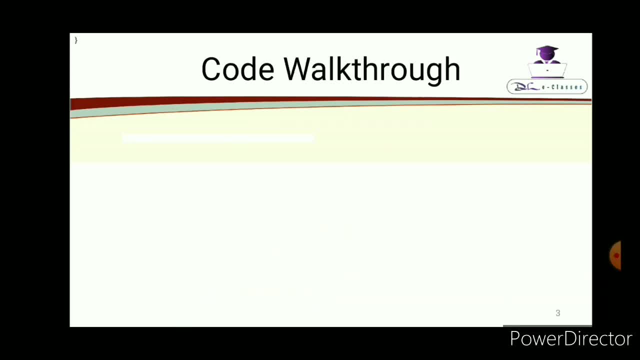 code workflow and the second technique is known as code inspection. Code workflow is an informal technique. So what is code workflow? Code workflow is an informal code analysis technique in which a module is considered for review after it has been coded, compiled successfully and all syntax errors. 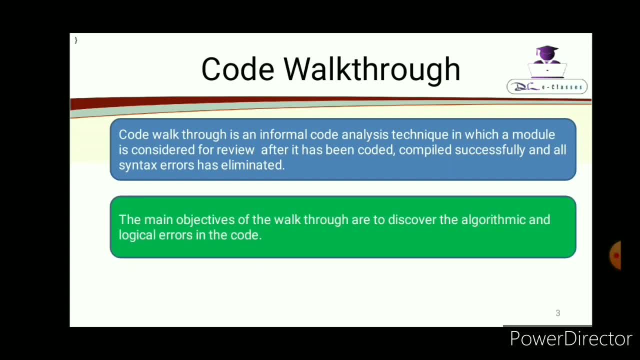 have been eliminated. The main objectives of the code workflow are to discover the algorithmic. and now what is algorithmic errors? algorithmic errors means: suppose you design a particular algorithm A for doing a particular task B, then if you are not intending, you have intended to obtain the goal B but you are not achieving. 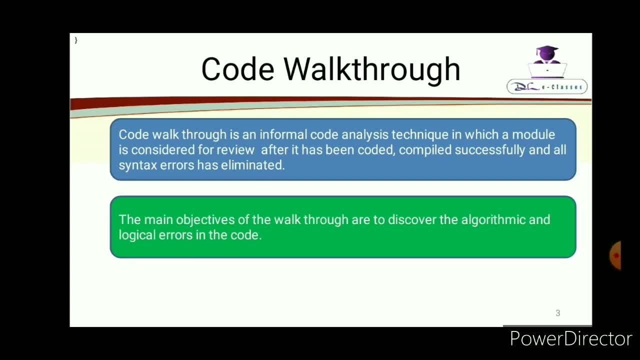 and there is no syntax error, but your output is not coming. that is an algorithmic error. now what is logical error? let us take one particular example. in the picture you see that there is a variable called I and your intention is to print values of I from 0 to less than 3, but by mistake you printed a. 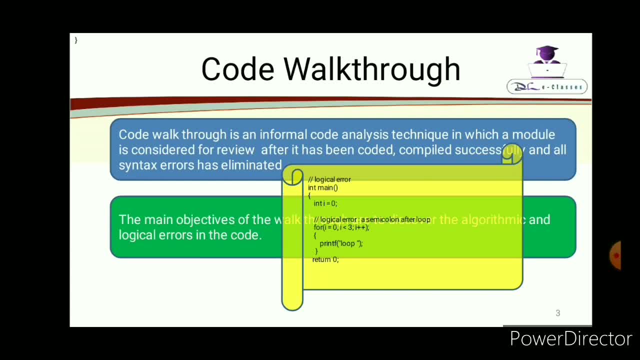 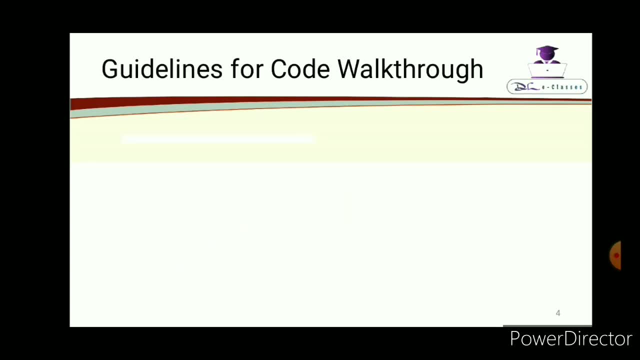 semicolon after the follow, then you are not intending the output. so it's one type of logical errors. now, although code workflow is an informal technique, the different guidelines have been proposed for doing the code workflow. now, what are the different guidelines? the team performing code workflows should not be 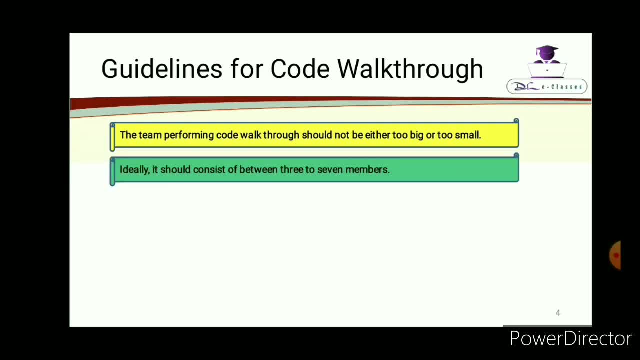 either too big or too small. ideally, it should consist of between three to seven members. discussion should focus on discovery of errors and not how to fix the discovery errors. so it should be very clear, in order to encourage cooperation and to avoid the failing of our engineers, that they have been 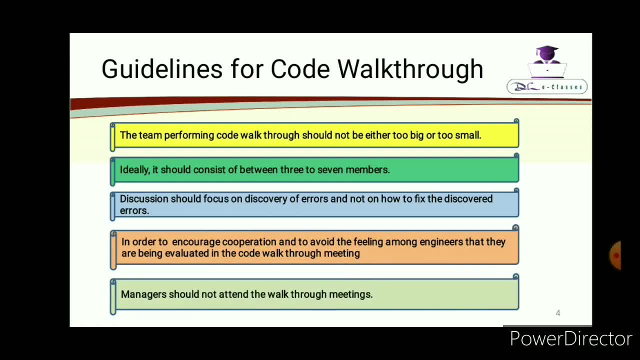 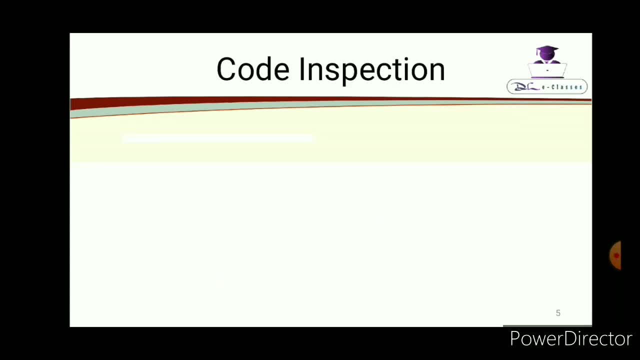 evaluated in the code workflow meeting. the manager should not attend the code workflow meetings, so that's why it is known as a formal technique. now, what is code inspection? it's a formal technique. we all know this. code inspection is a formal code analysis technique. during code inspection, the code is examined for the presence of certain kinds of errors. now, what are the? 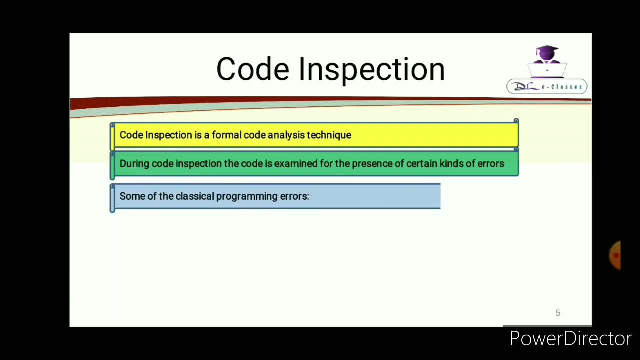 different types of errors. those are known as a classical errors. some of the classical programming errors are use of uninitialized variable. for example, you see you have used a particular variable, I, and that variable is not declared. so it is one kind of uninitialized variable errors. jumps into loops. you see in the picture design a particular program and by 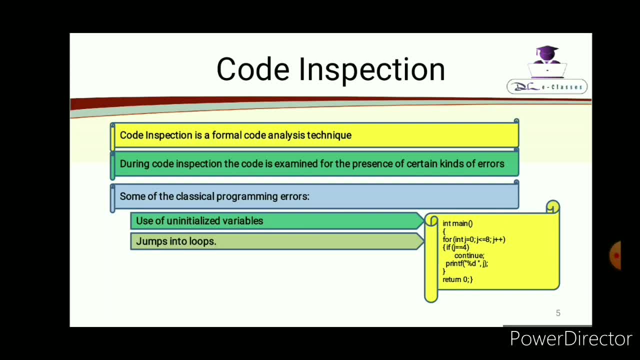 mistake. you have continued a loop, then you are not getting the outputs now non-terminating loops. it can be another errors in the picture. you see that you have declare a particular for loop and it is not terminating while the kind of loop never ending. then incompatible assignments, suppose we. 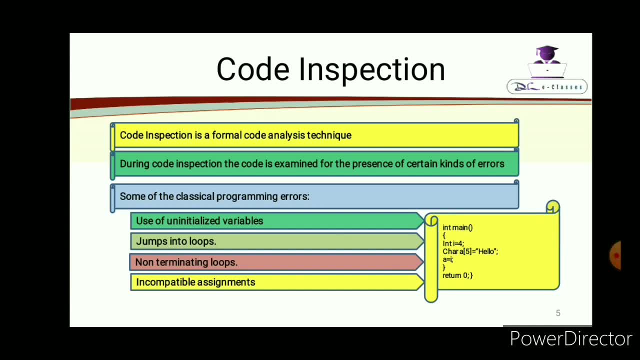 have. there is a variable called I. you have assigned a value of a, the character arrow. take the array hello and you are assigning yellow integer to character. so it's a problem. another error, or classical error, is this error indices out of bounds. sometimes this type of errors can be. 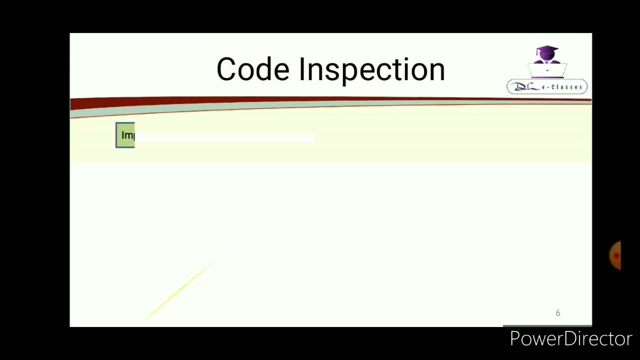 you can see the error index is out of bounds. sometimes this type of errors can be. you can see the error index is out of bounds. sometimes this type of errors can be done, can be happened, don't? some other remaining classical errors are just like improper storage, allocation and the allocation mismatches between 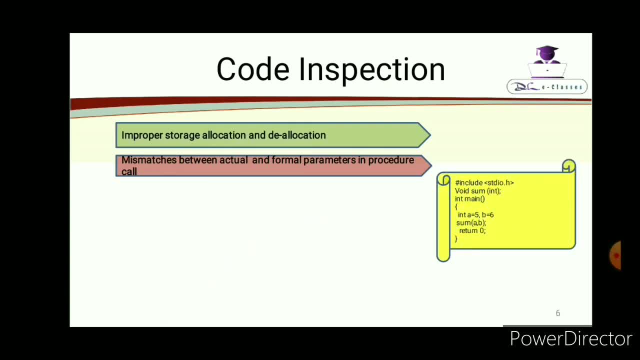 excellent form, it's missing. focus on. other errors can be use, use of incorrect logical operators or incorrect precedence among the operators. for example, suppose your intention is that there should be an end operator between a and b in the picture, but you have, by mistake, one ampersand symbol is given, so it's just like b2s or end. 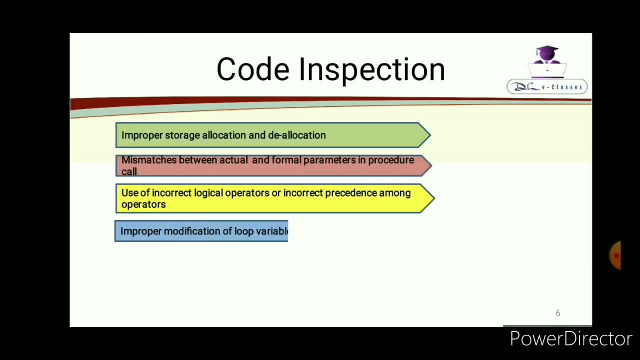 operator. so it's a problem, so it's an error, so it's not intentional. actually. another kind of error is improper modification of loop variables, so it's also one type of classical errors. for example, you have in the picture you have seen that given values, say i is equal. 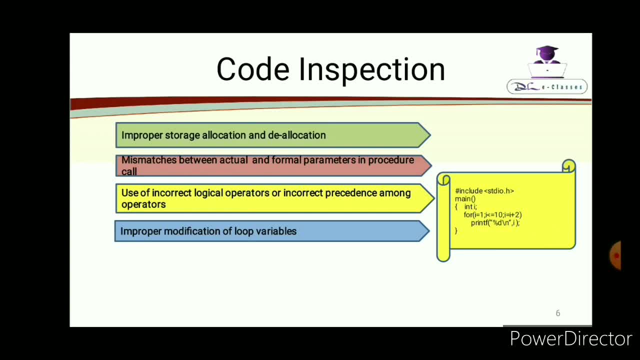 to 1, 2, 4. you have seen that the improper modification is done. your intention is to print the values from one to ten continuous, but by mistake or by unintentionally, you have given it a, even two increments, so you are not getting down. so it is not actually syntax errors, but it's. 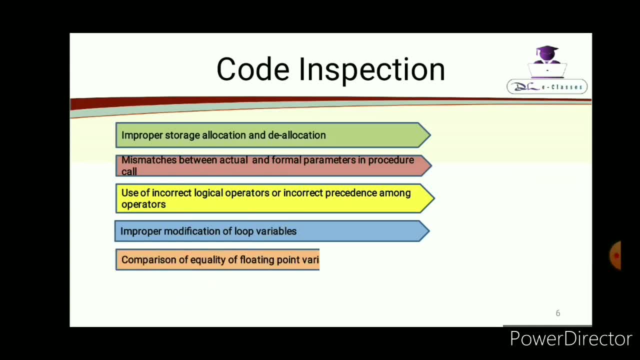 improver modification of the low variables. so another classic error may be comparison of equality of plotting point variables. for example, suppose there is a variable float, a variable 3.4 values. there is another variable, double b, equal to 3.4, although the values are plotting point. 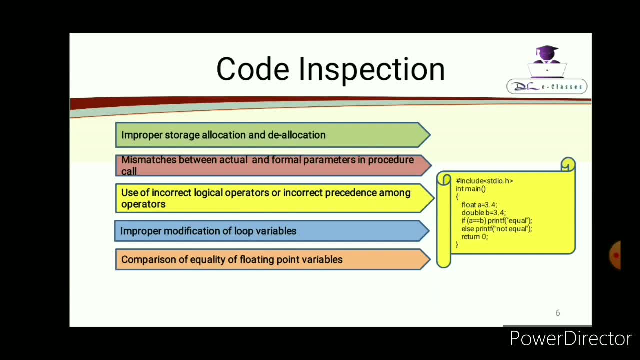 they are same when you're comparing, it is saying that they are not equal. so it should be not intentional errors, so it should be. you should keep in mind. so this type of errors, of classical errors you have to. main aim is aiming the code, inspection is to detect this type of errors. now, finally, uh, 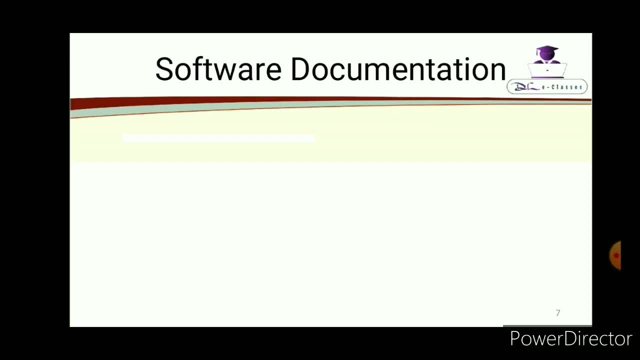 what is the document? when we are talking about a coding process, documentation is a very important thing because the documentation always plays an important role in the software development process. so when you're talking about the documentation, that means software documentation. they are classified basically to two types. uh, now, what is software documentation? a? 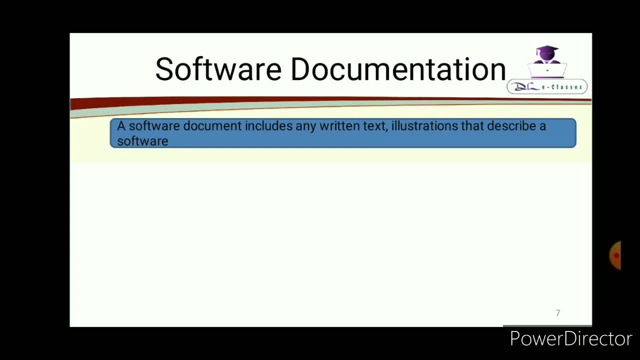 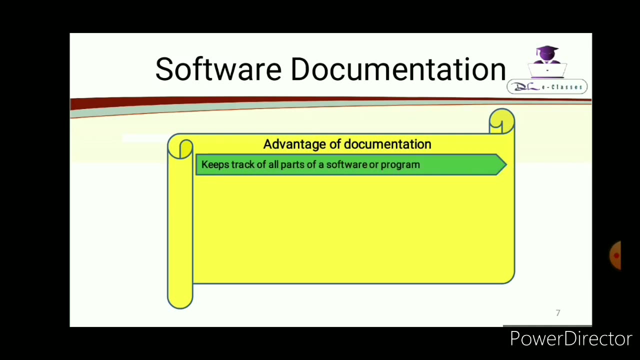 software documentation includes any written text illustrations that describes a software. software documentation is very crucial in the overall software development process. now there are what? uh, various type of advantages. now, first advantage: uh, there are many advantages. let us take some of the advantages. the advantage is that it keeps tracks of all parts of the software. 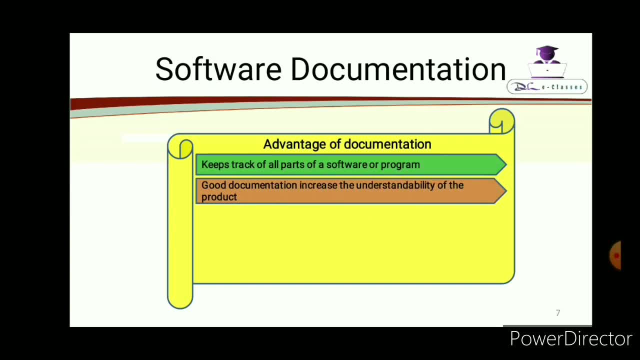 development program. good documentation increase the understandability of the product. reuse the effort and time required for maintenance. improves overall quality of the software of the product. helps to handle the main core turnover problem effectively. so what is the main core turnover problem? suppose you have developed a particular software under development, a particular 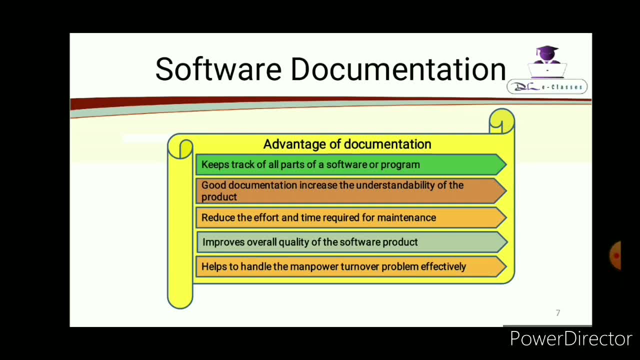 software. your members are five software programmers are doing uh during the. in the meantime, suppose one or two programmers left, then you have to recruit another people in place of them, and if you maintain proper documentation then they can start right from the beginning. the right from the beginning means right at the time of they left. whatever, whatever the development, 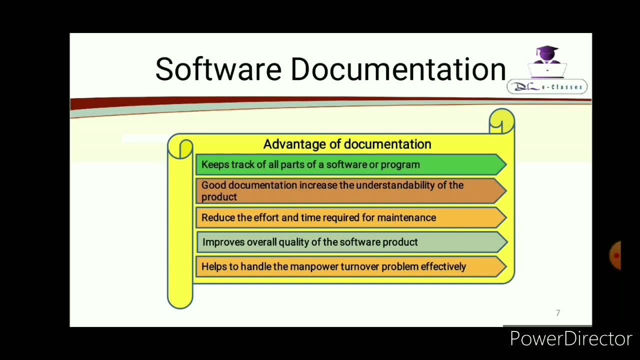 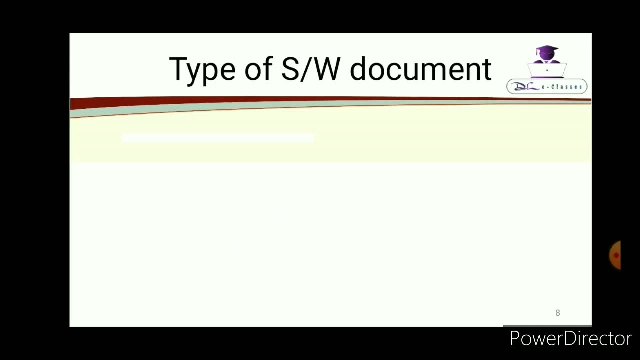 is over. from that point, of that point onwards development can be started. so documentation plays a very important role. so this type of problem handling is one of the main power turnover problem. now, what are the different types of software document? software documents have different classification, but rather we can classify into two main categories. 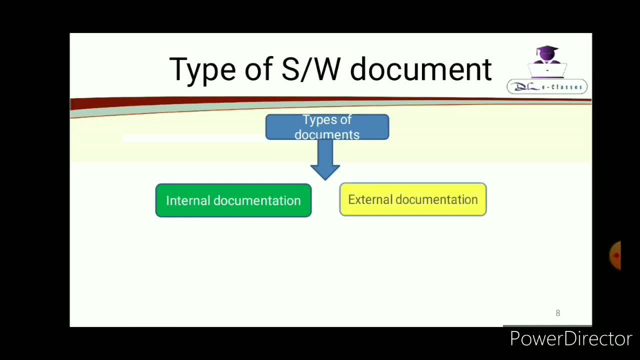 the first one is internal documentation, second one is external documentation. so internal documentation actually means the comment which you are, which the programmer writes inside the code. for example, you see, there is a program to find out whether the number is given, whether number is odd, or even the program is written in c. now the comment line you have seen.